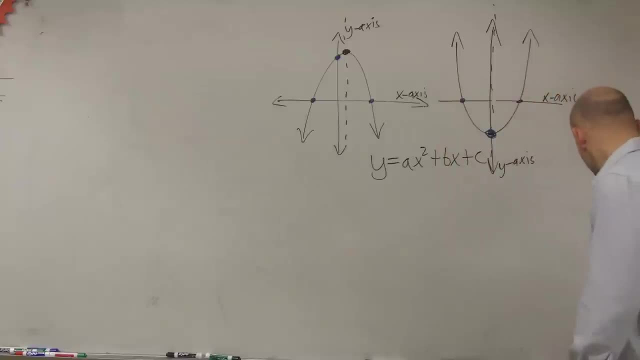 Okay, So let's go ahead and talk a little bit about the blue, Okay, And actually you know what? Yeah, let's go and talk about: eh, let's change this up, Let's make it red for the x-intercepts, OK. 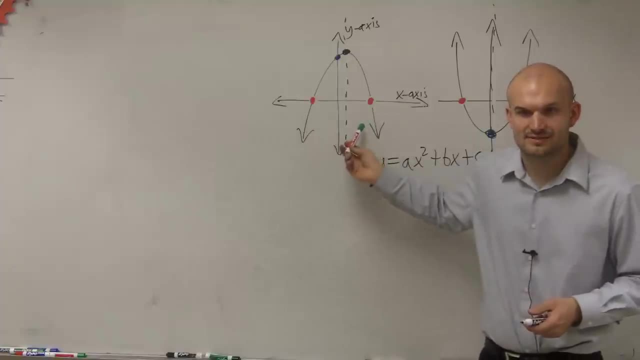 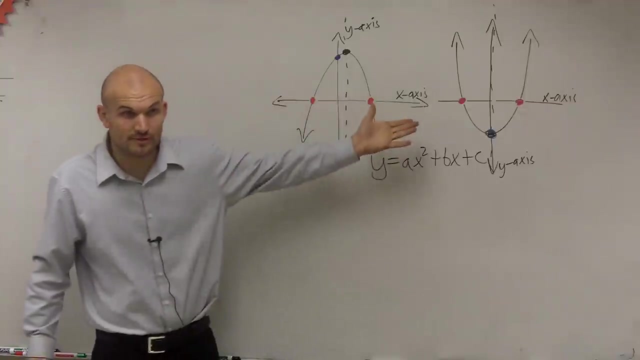 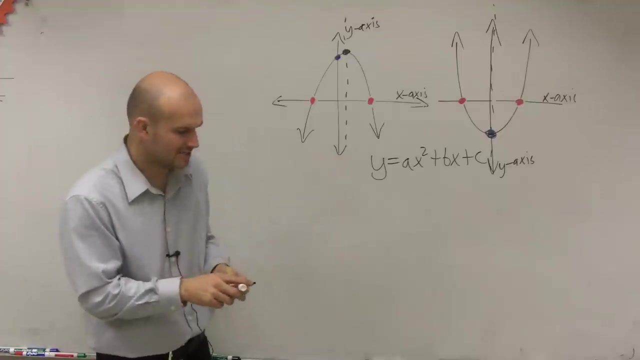 So when the graph crosses, when the graph crosses the x-axis, those are what we call our x-intercepts, right, x-intercepts? OK. Now here's one thing. I want you guys to understand: The x-intercept. what is the y-value? right? 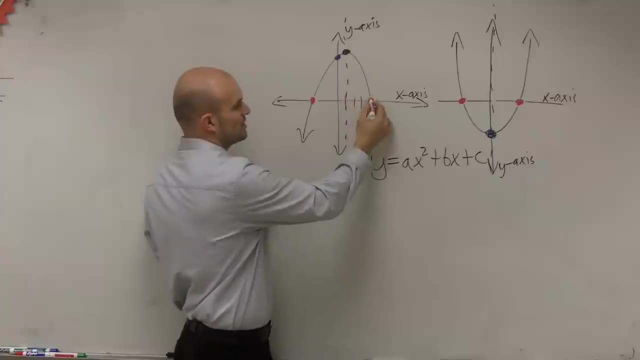 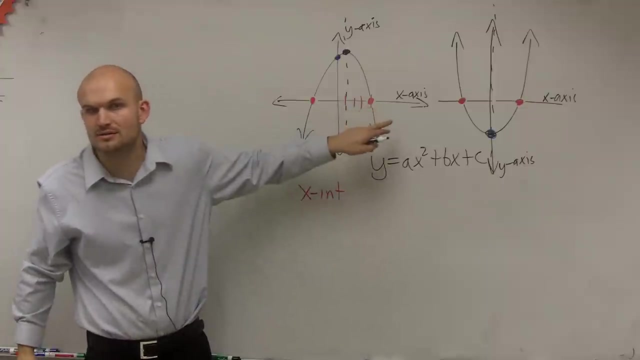 You guys know, when we have tick marks, you go over 1, you go over 2, you go over 3,, you go over 4, right, So this point is 4 comma. what? What is the y-value at that point? 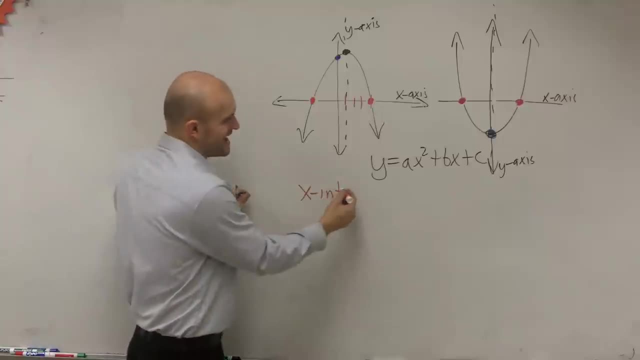 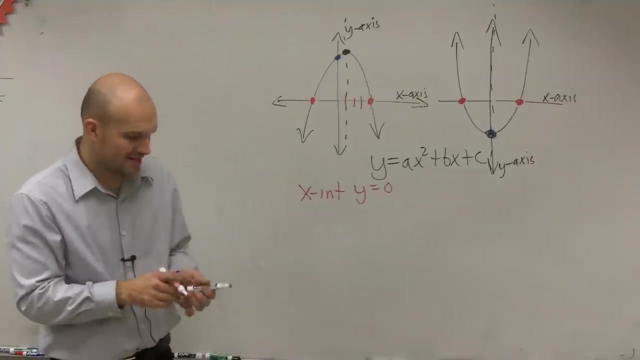 0.. So what we can say, what you guys are going to write down is: x-intercept is when y, y equals 0, OK, Then let's go and take a look at the blue points. The blue points are where the graph crosses the y-axis. 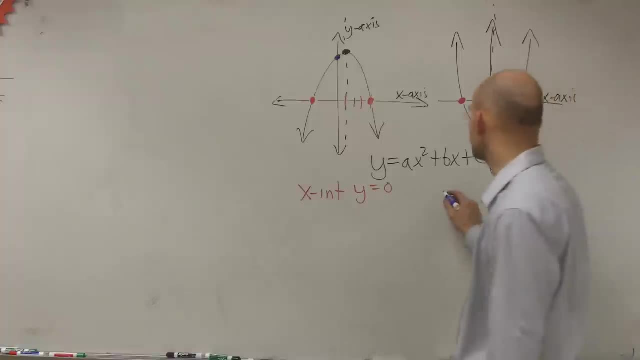 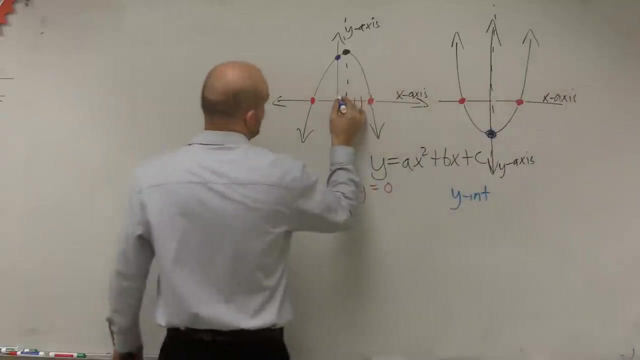 So we could say those were the blue points where they crossed the y-axis. we call those the y-intercept And the y-intercept, if you look at this. let's look at this point, which would be at like 1,, 2,, 3,, 4,, 5,. 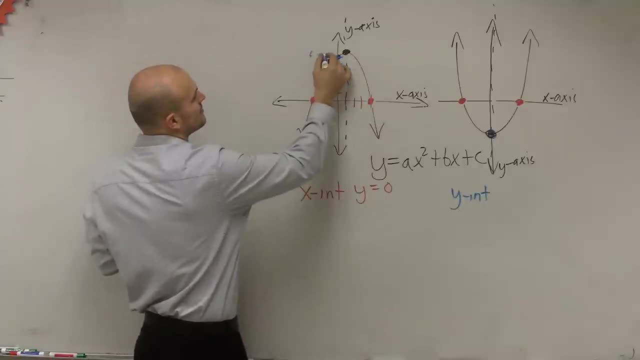 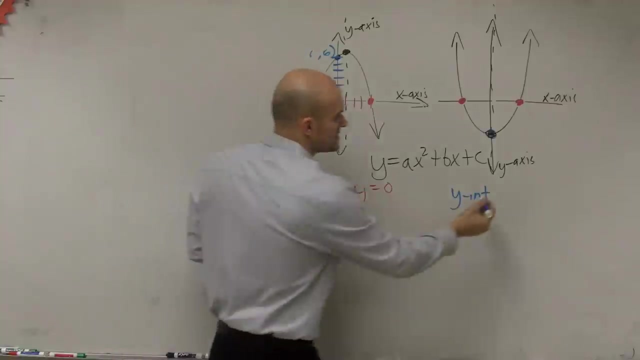 6. So this point is at 0.. What is the x-value when the y-value is at 6? 0. 0. So you could say x equals 0. And let's write in that point for you guys to help you out. 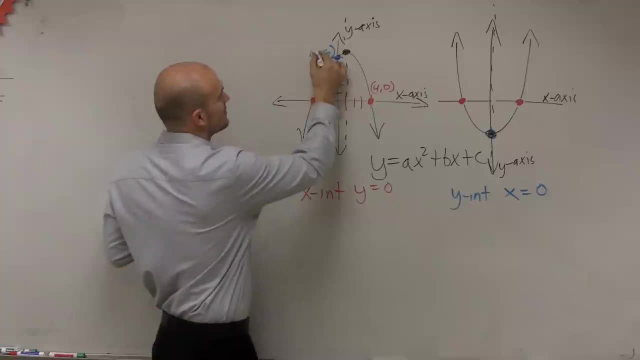 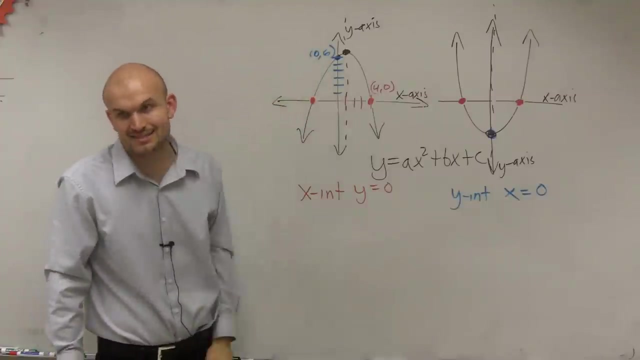 Do you guys see that when the graph crosses the x-axis, the y-value is 0?? When the graph crosses the y-axis, the x-axis, The x-axis, x value is zero. Do you guys see that? Yeah, kind of opposite. So let's go and look at. 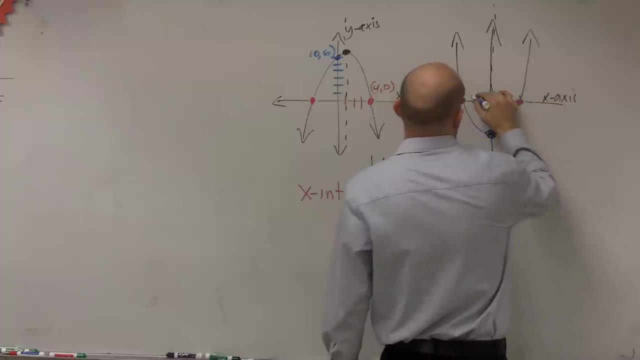 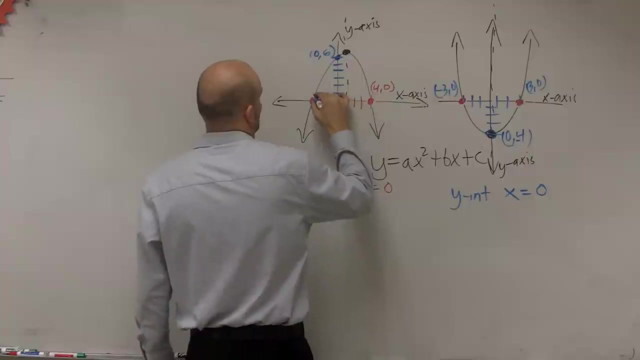 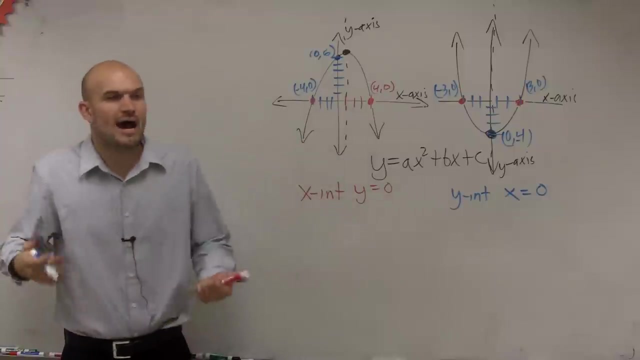 these two points. So this one would be zero comma four, negative four, and this one is three comma zero and negative three comma zero. Okay, so you guys can see how these points work, right? So how do I find? if I give you an equation, how are you going to? 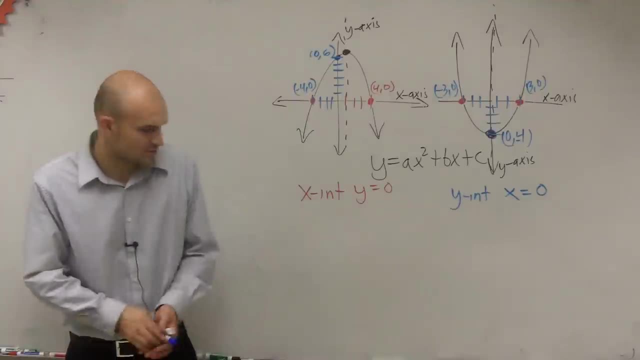 determine, then, what the x and y intercepts are. Okay, so let's go and take a look at a problem. I'll just give you a fairly basic problem and we'll just work from it from there. So this new equation is not going to have any resemblance to these two. So let's 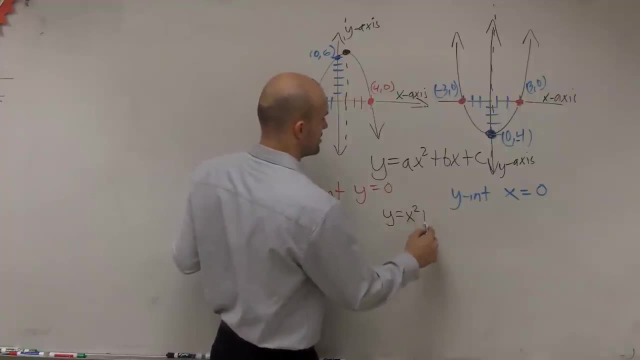 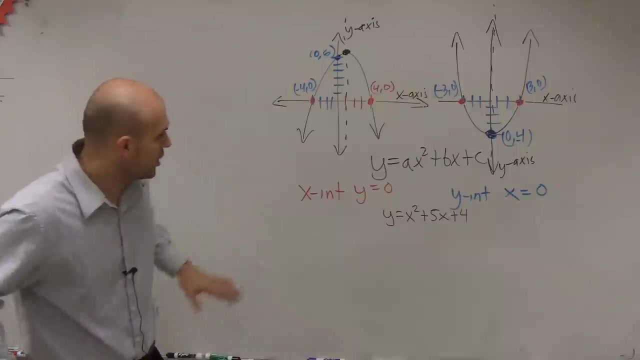 say, I say y equals x squared plus 5x plus 4.. And I say: tell me what are the x and the y intercepts? Okay, Okay, So to find the x intercept. that means y equals zero. So you're going to put a zero in for. 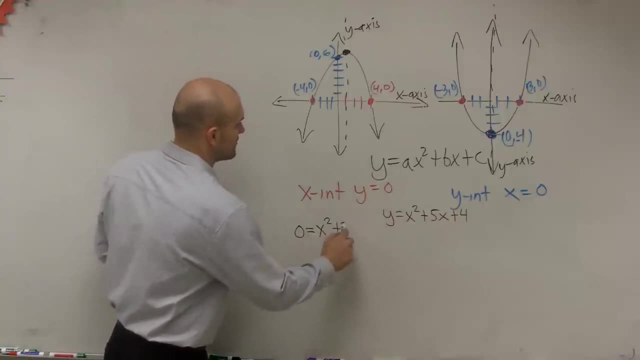 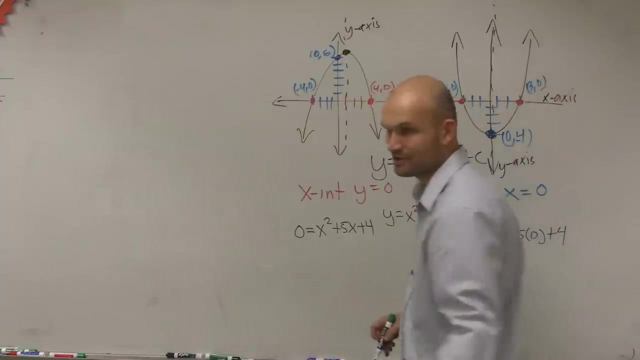 y Zero equals x squared plus 5x plus 4.. To find the y intercept, you're going to put a zero in for x. So you do: y equals zero squared plus 5 times zero plus 4.. Does everybody kind of see the difference? The x intercepts are when y values equal zero. So you put a zero. 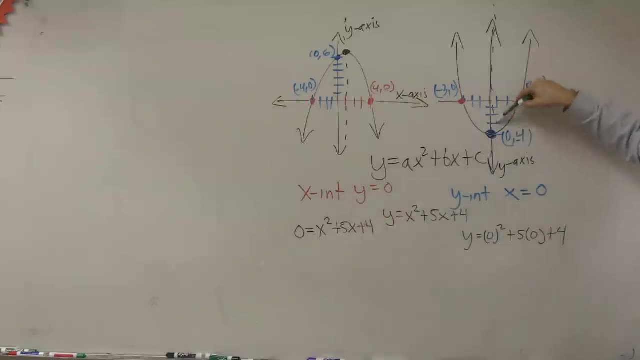 in for the y. The y intercepts are when the y intercept is when x equals zero. So you put a zero in for x in the equation, Kind of make a little sense. Yep, How it follows. Everybody does that. Okay, So now we just need to solve for the other variable. I like doing the y intercept. 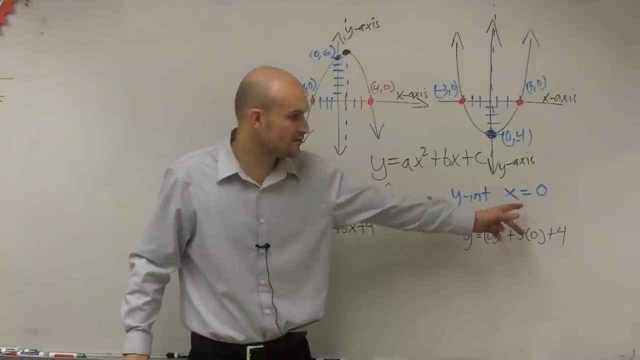 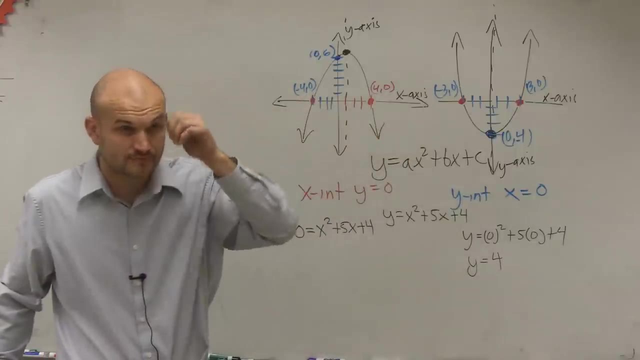 because this is pretty easy: Zero squared is zero plus 5 times zero is zero plus 4.. Therefore, the y intercept for this problem is: y equals 4.. Yes, When you first grabbed them in there, wouldn't it be negative? 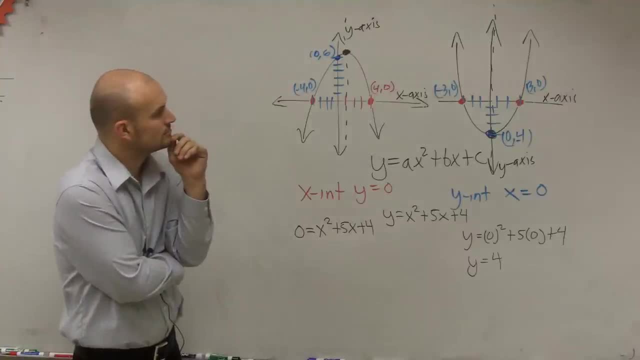 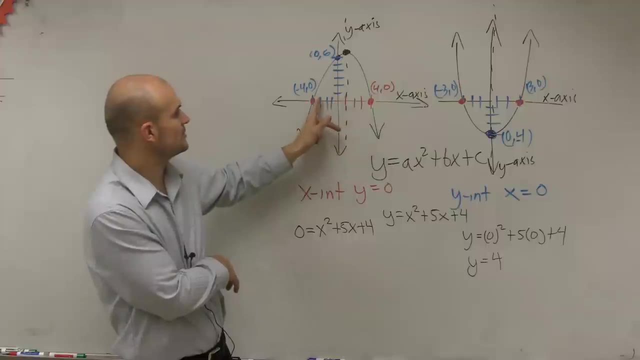 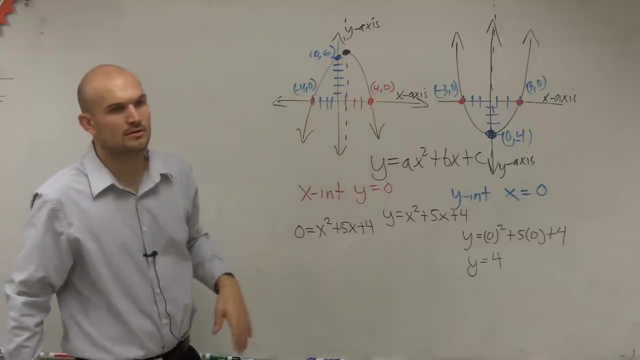 Here. No, I marked it out as 1,, 2, 3, 4.. It's not very scalish, but yeah, I put four tick marks: 1, 2, 3, 4.. It's not supposed to be. it's just supposed to be a reference. It's not supposed to be. 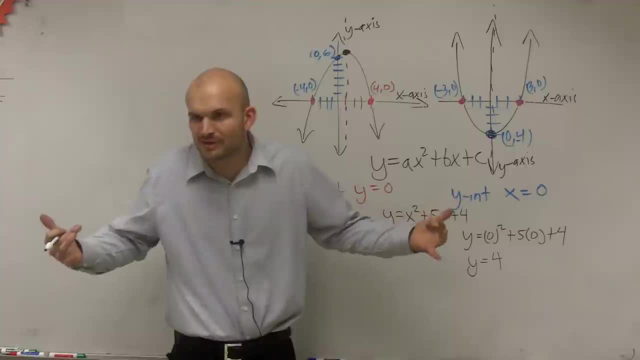 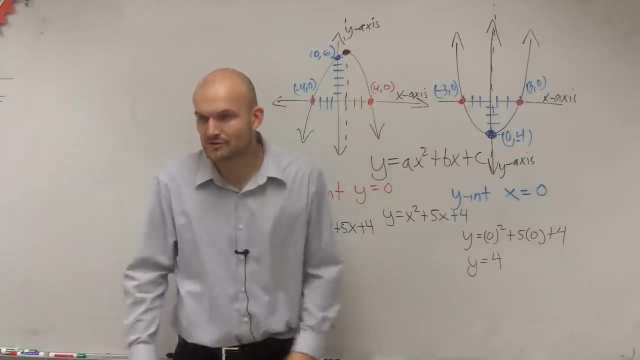 exact, Okay. So y equals 4.. That one's pretty basic. right Now. you guys remember why we spent like three weeks factoring, Okay, Okay, Guess what. Here's where the factoring part comes in. How do you solve for x when? 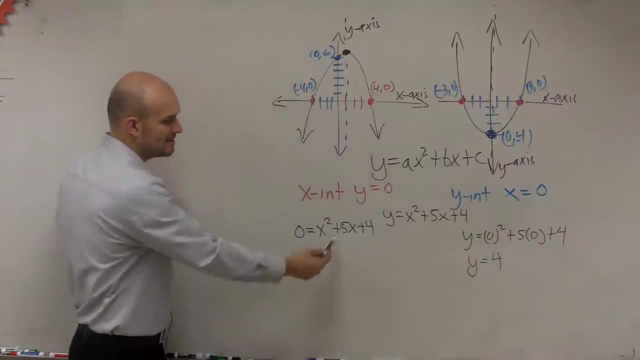 you have two of them Here, was pretty easy, You just simplified. But now guess what you have to do: Tractor. You have to do what Factor Tractor. So zero equals x plus 4 times x plus 1.. Now remember why did we solve by?